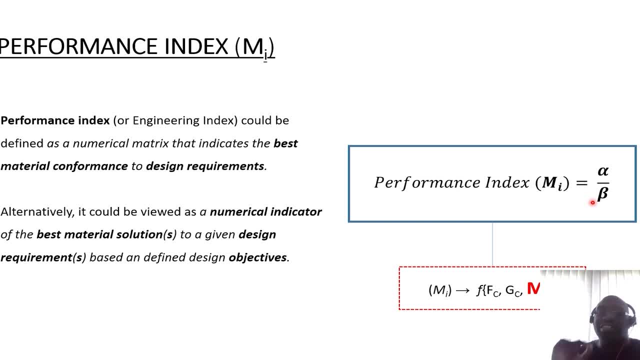 But the key element here, when it comes to CES, is the material constraint, And this is where it becomes important to have a good understanding of what are the desired characteristics that you seek in the material. So we're going to look at this example where we've been given a bicycle frame. 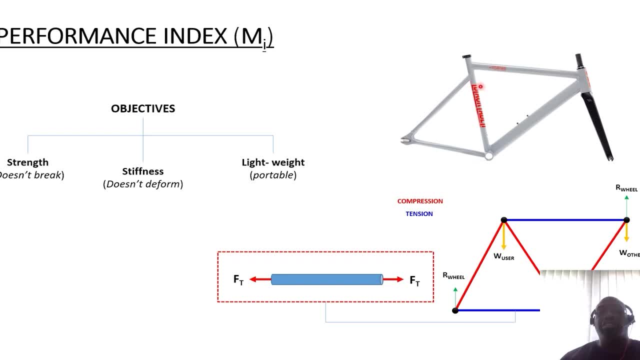 So I've modelled the bicycle frame to a truss to look at the loading conditions and to look at which elements are being subjected to either a compressive and or tensile load. In terms of the objectives, then, it's very important that you make clear what your objectives are. 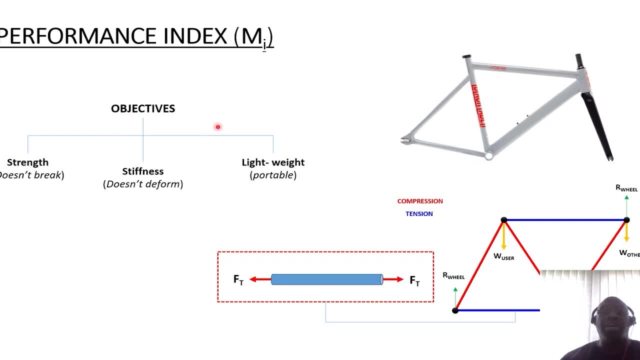 What are you trying to achieve? you know from this exercise. So we're going to look at this example where we've been given a bicycle frame. So we're going to look at this example where we've been given a bicycle frame. What are you trying to achieve? you know from this exercise. 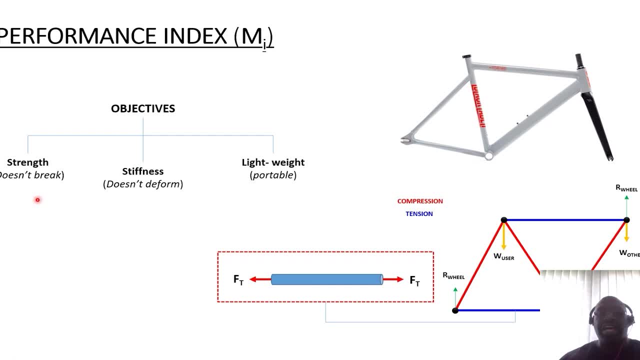 So, in terms of this bicycle, we're looking at its strength, So we hope to select a material that does not break when loaded. We're also looking for material that is quite stiff, so that it doesn't deform or warp out of place, But at the same time, to improve product performance, we expect it to be quite light. 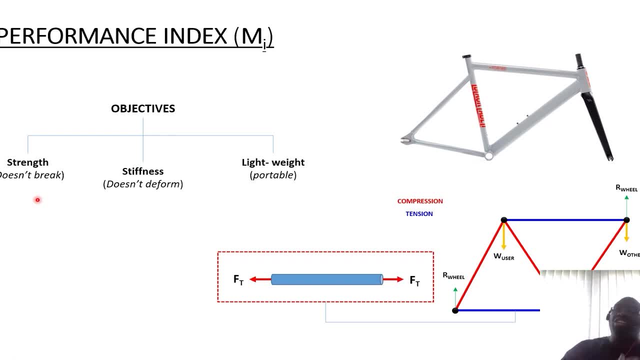 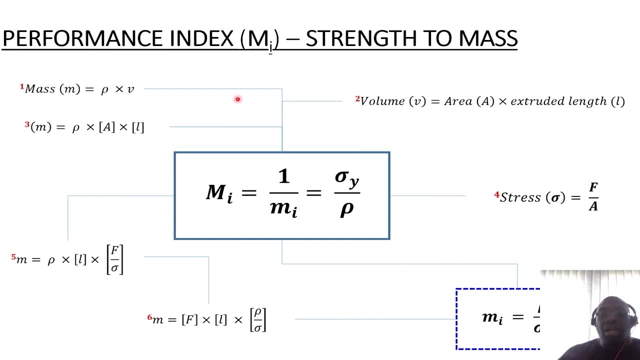 So the lesser the weight, the easier it is for it to generate the needed energy To be displaced faster. So these are the objectives in identifying the best material for the bicycle frame. So when it comes to the performance index, I'm not really going to go. 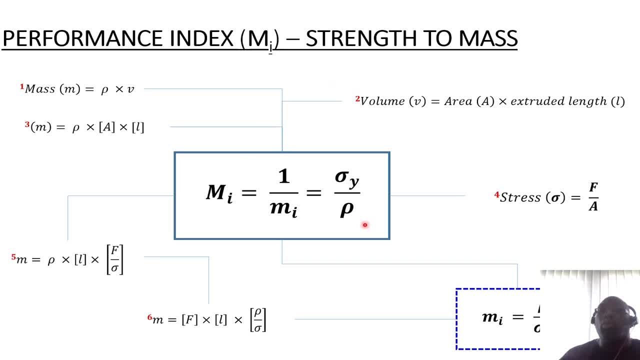 too much into the mathematics of this, because it's not really important All that. all this information has been listed in CES, So it just comes down to having an understanding in terms of what the operational or functional requirements are for your design. But just to illustrate, this, metric is an amalgamation of mass equation, which is basically: 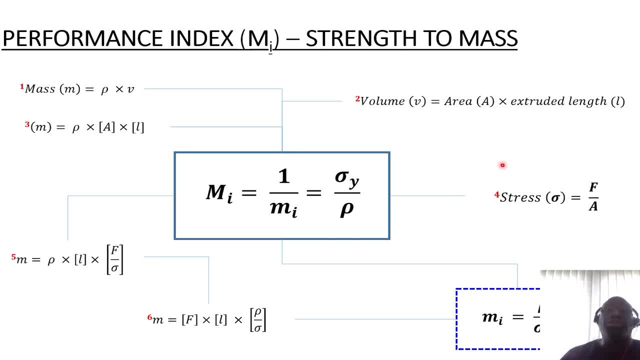 a transposition of the density formula and the stress equation. So once these are amalgamated, they're then compartmentalised in terms of what the functional variable is, what the geometrical variables and what are the variables that links to material. When it comes to CES, the focus is to maximise the index to indicate the best material. 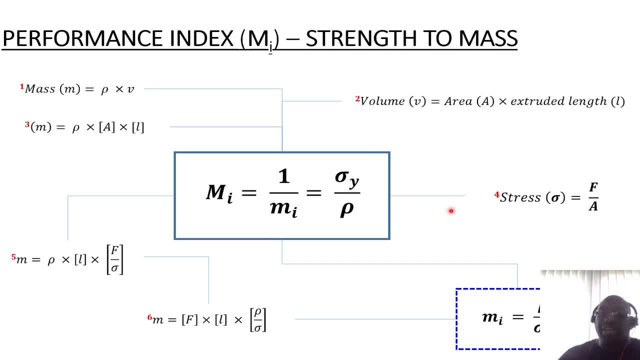 that can be considered for a given application. So, in terms of deriving the metric, it will give you the content in terms of minimising the metric, But to use CES you have to look at maximising the index to identify the best materials that provide the best conformance to your design requirements. So this is for strength to mass. So the index when? 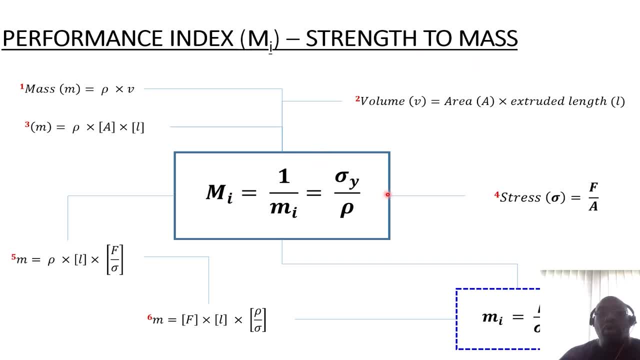 we're looking at strength to mass would be sigma y. So sigma y characterizes the yield strength in this context, and rho represents the density. So the higher the density, the smaller the metric, because you know you're increasing the mass, So for this to become larger, to give you an 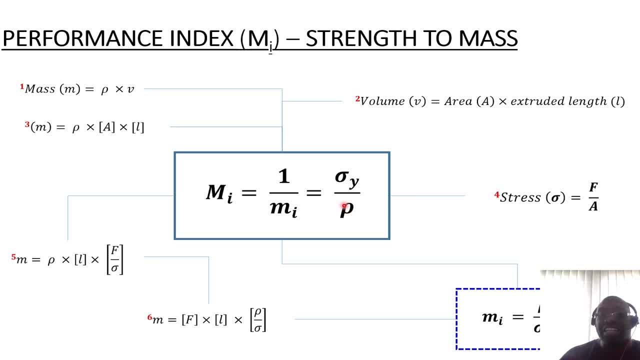 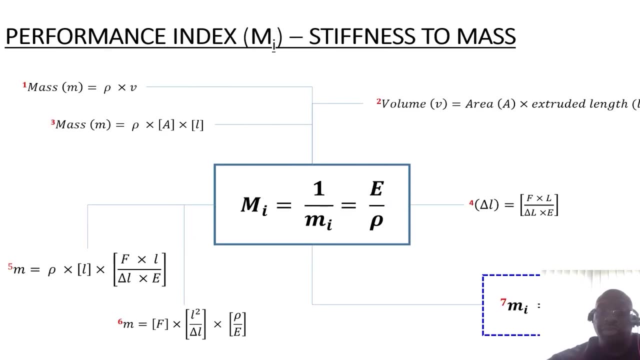 indication that you are reducing the mass, then the density needs to be smaller. So that's a simple interpretation of this. There you go. Similar to the previous, we can also look at the stiffness to mass. So we're looking at how much the material can withstand deformation, but at the same time also looking at material that exhibit. 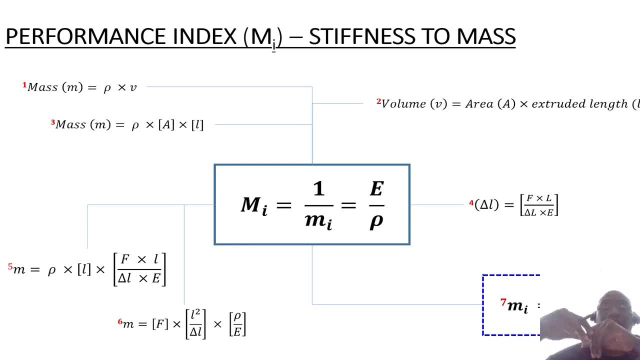 considerable lightness to ensure that it doesn't impede the performance of the bike when work is placed in to move it from one point to the other. I think, naturally, you know, everyone would think you know- the denser the material, the better it is to withstand deformation. However, the more mass the structure contains, 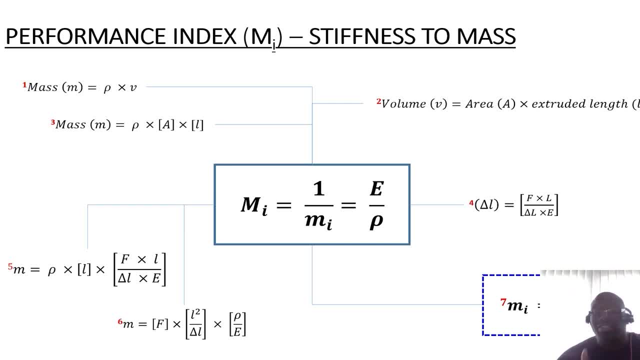 the more more work will be required in moving or displacing the bicycle from one point to the other. So it's important that, while we're also looking at you know, material that exhibit you know good stiffness characteristics, we also need to look at material that are: 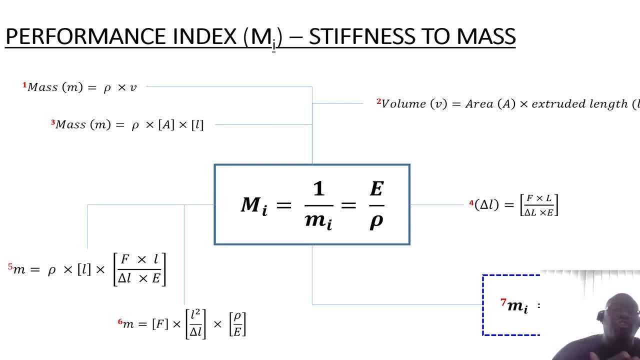 significantly lighter to enhance the performance of the product, in our case the bicycle. Similar to the previous example, this is just an amalgamation of the density equation to that of axial deflection. So once the two equations are merged, it's just a question of partition or compartmentalizing the functional constraint.